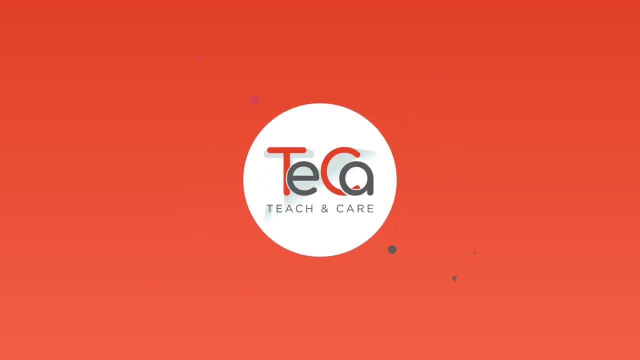 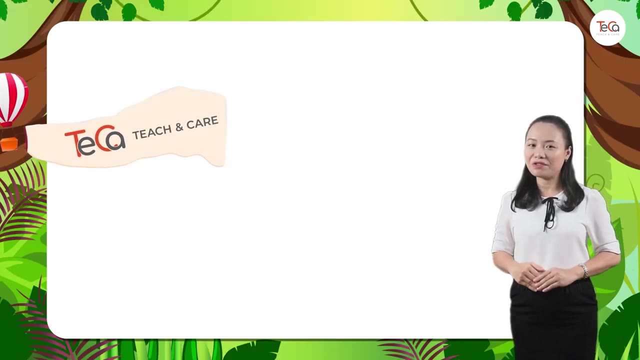 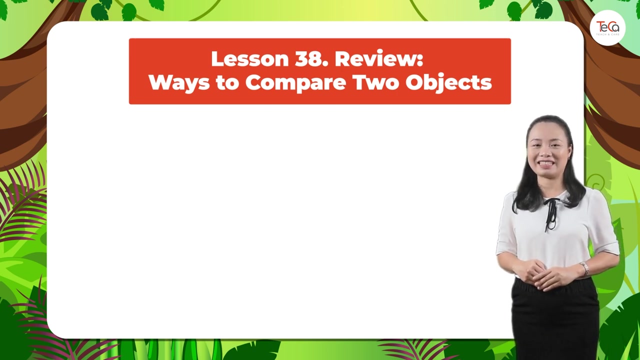 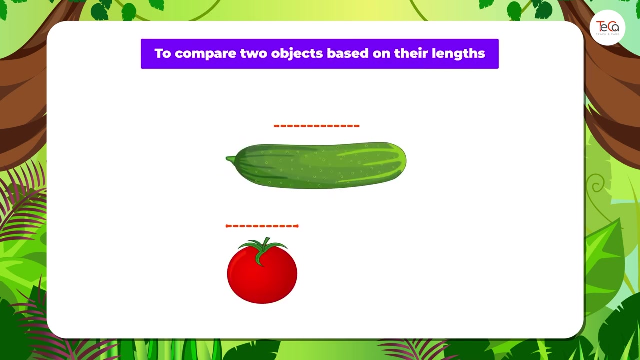 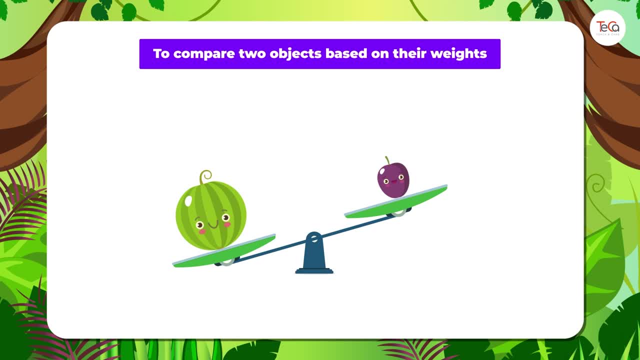 To compare two objects based on their heights, we say taller, shorter. To compare two objects based on their heights, we say taller, shorter. To compare two objects based on their heights, we say taller, shorter. Based on their weights, we say heavier, lighter. 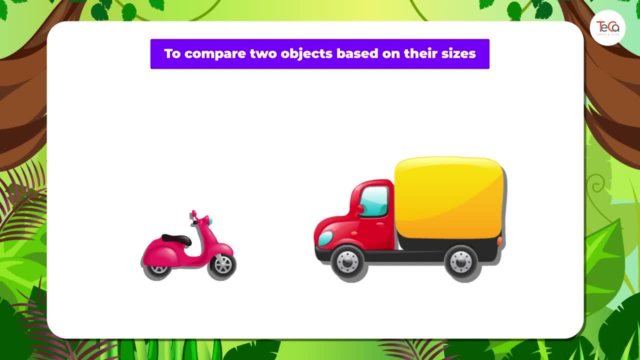 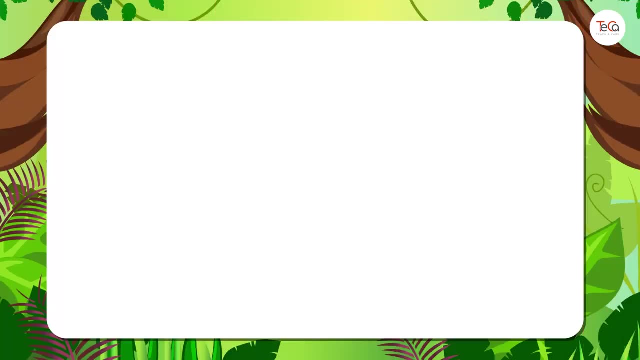 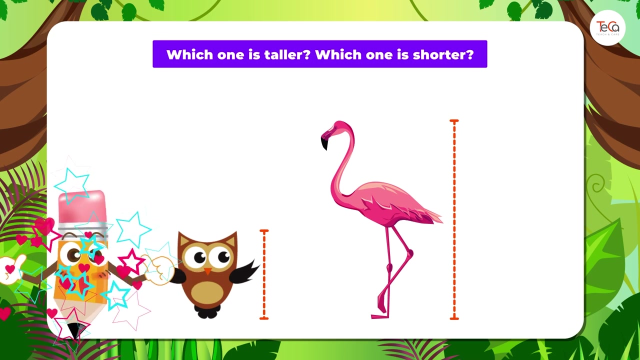 To compare two objects based on their sizes. we say bigger, smaller. Now let's practice. Tell me Which one is taller, Which one is shorter. Great, The flamingo is taller Or the owl is shorter. Tell me. 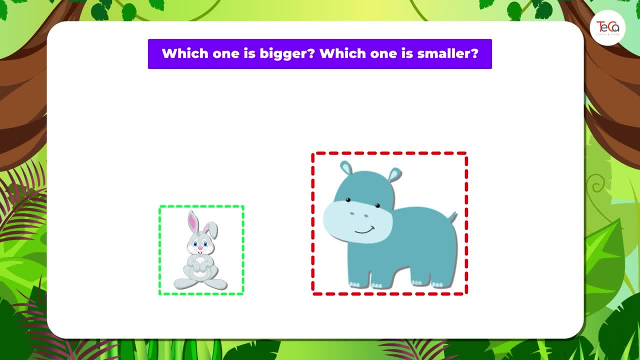 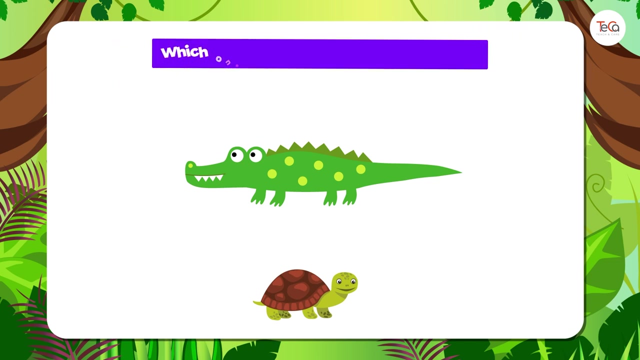 Which one is bigger, Which one is smaller, Which one is smaller? Super, The hippo is bigger Or the rabbit is smaller. Tell me Which one is longer, Which one is shorter, Which one is shorter? That's right. 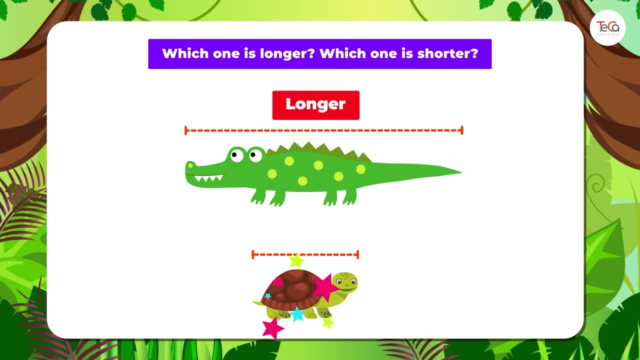 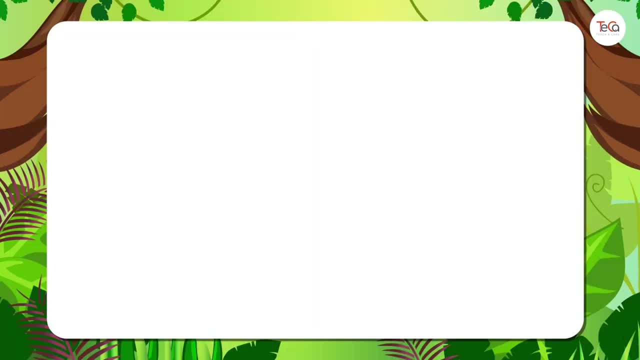 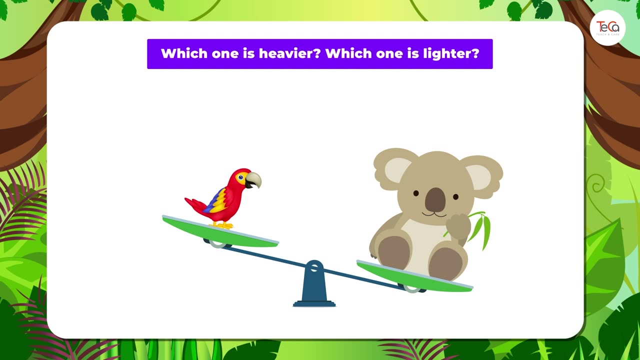 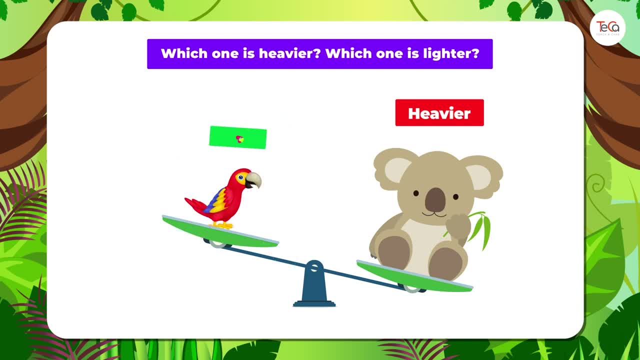 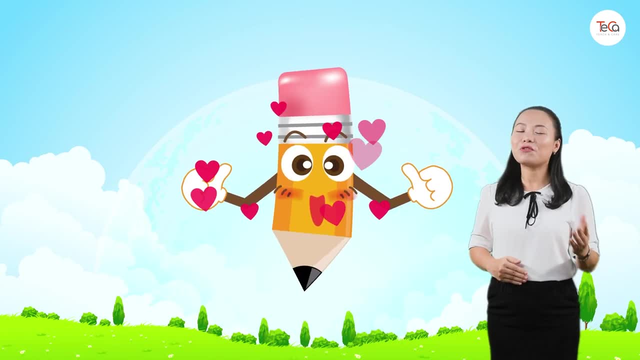 Good. Good, Or the parrot is lighter. Great, You've finished. Bye for now and see you soon in the next lesson. 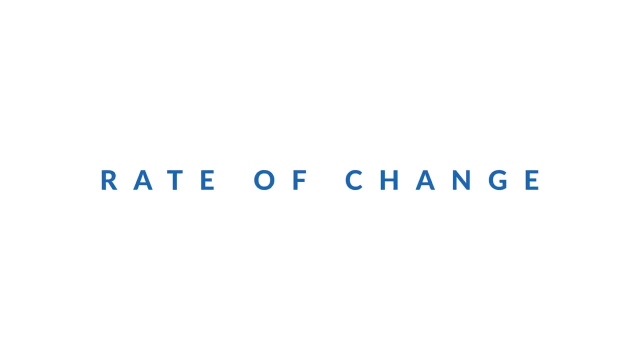 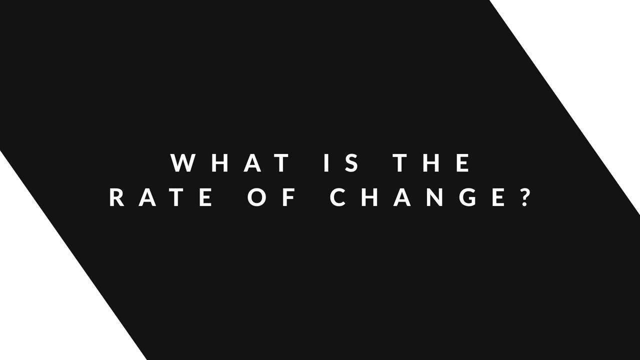 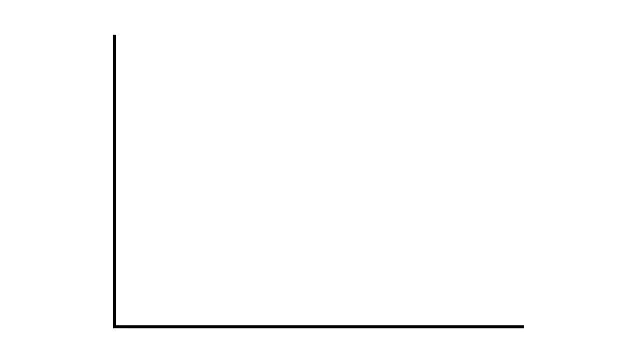 Rate of change. Let's get you from 0 to 100.. What is the rate of change? Simply, it's literally getting you from 0 to 100, or also commonly known as rise over run. Let's assume that we have a graph and on this graph we have a line that goes forever. As a side note, this line is also known as a regression line. 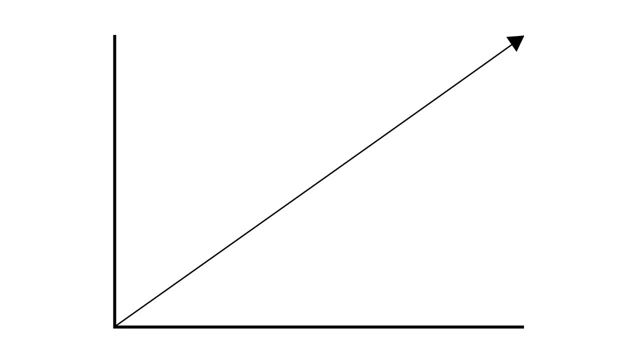 Now let's assume that we have a point that we will mark with dotted lines. The question that we are answering is: how do we get from 0.0 to 0.100? This can be calculated with a simple formula. What is the formula to calculate the rise over run? 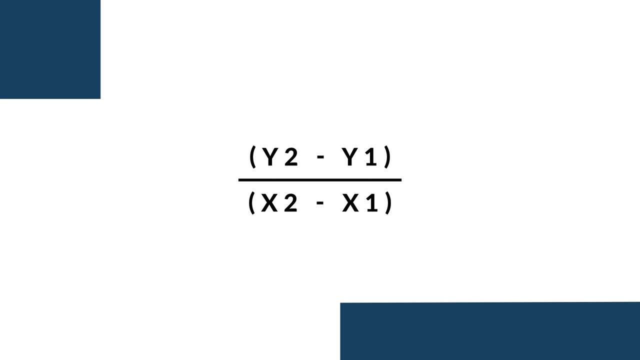 You can take y2 minus y1 and divide that by x2 minus x1.. Let's assume that we have a graph and on this graph we have a line that goes forever. As a side note, this line is also known as rise over run. 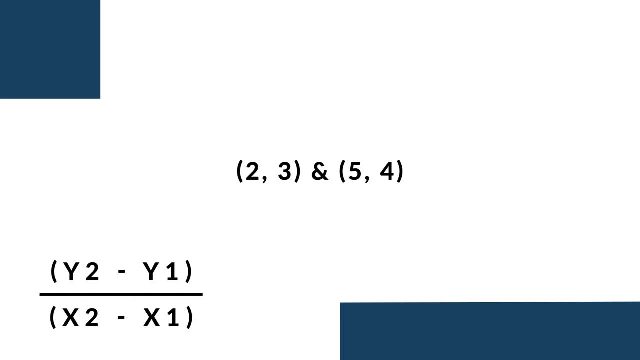 Let's assume that we have the points 2 and 3, and then another pair of points, 5 and 4.. Plugging in the numbers to the formula, we get 4 minus 3 over 5 minus 2.. As you can tell, 0.1, which is 0.23, is on the right side of the formula. 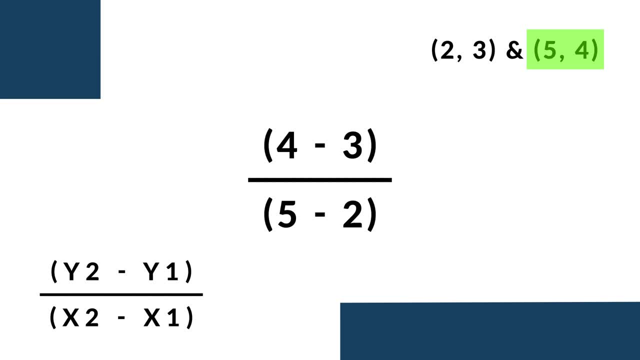 And 0.2, which is 5.4, is on the left side of the formula. If we do the math, we know that the result is 1 over 3.. That is the rate of change for these two given points.